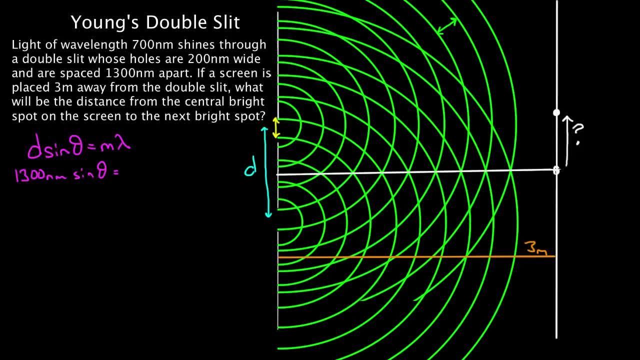 I'm going to worry about the angle from. Here's my center line, From there to the point I'm concerned with is this first bright spot past the center point. So that's the angle I'm concerned with. This angle right here equals m. What should m be? Well, this is 0. Should I put 0?? No, because I don't want the angle to the center one, I want the angle to the first one over here. So this is m equals 1, the first order bright spot. constructive point. times the wavelength. 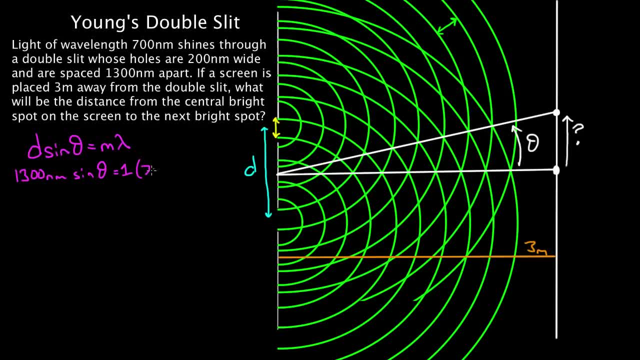 What's the wavelength? The wavelength of the light we said was 700 nanometers. Now you might be wondering: wait a minute, what about this 200 nanometer wide piece of information? Do we have to use that? No, we don't. In fact, that does not play into here. The only time that this spacing is important. it's not going to change your calculation. You just need the spacing to be small. small enough that you get enough diffraction, that you get a wide enough angle of diffraction that these two waves will overlap. 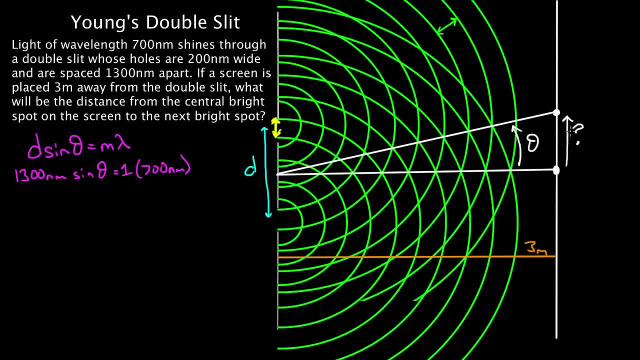 Significantly enough that they'll create the interference pattern that you want to see over here to a degree that's visible. Okay, but we don't need it. We don't even have to use that one in our calculation, Alright. so we calculate the angle. Here we go. So I'm going to find sine of theta and I'll get that. sine of theta equals 1, is just 1, so I divide both sides by 1300.. I get 700 over 1300.. The nanometers cancels nanometers. As long as I'm in the same units, it doesn't matter. 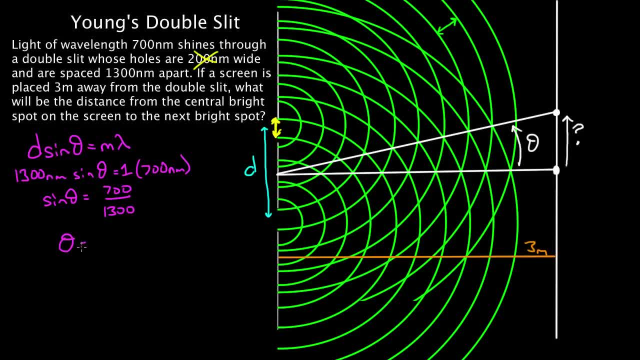 I'll solve this for theta. How do I get theta? I've got to use inverse sine of both sides. So the inverse sine of sine theta is just theta and the inverse sine of this side gives me 32.6 degrees. That's what this angle is right here: 32.6 degrees. but that's not what I was trying to find. What I'm trying to find is this distance. 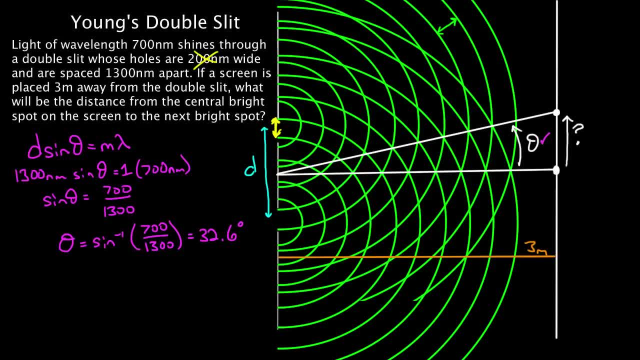 This angle. So how do we do that? Well, this side, this side right here, I'm going to call it delta y, because it looks like it's a vertical distance- This is the opposite side to that angle. That's the opposite side. We know the adjacent side. This adjacent side, we were told, was 3 meters away from the screen. 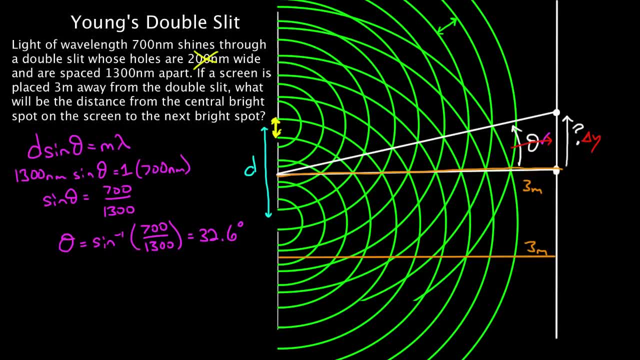 The screen was 3 meters away from the double slit. And how do we relate the opposite side to the adjacent side? Shoot, I know how to do that. Tangent theta equals opposite over adjacent And our opposite is delta y over 3 meters in this case. So if I solve this for delta y, I'm going to get delta y equals, multiply both sides by 3 meters, times the tangent of theta Theta we solved for right here, 32.6 degrees. 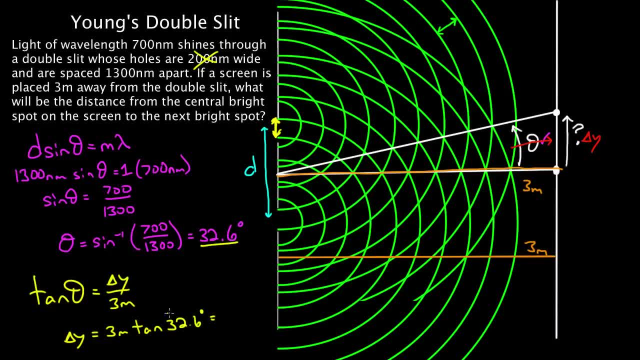 And if you multiply all that out, you get 1.92.. 2 meters- That's how big this would be. From here, center point to the next bright spot is 1.92 meters. That's how you solve this problem. 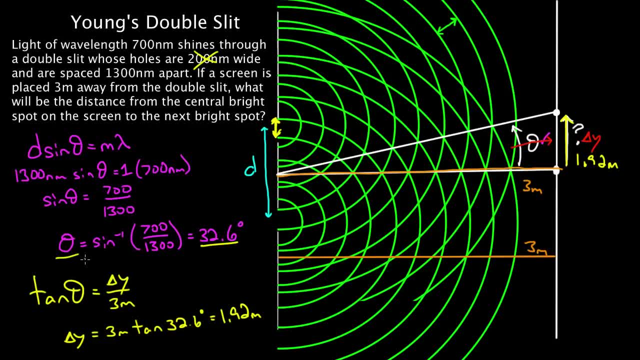 You've got to use a little trigonometry. once you get your angle, You've got to relate it to a distance vertically on the screen, And this is a common problem using Young's double slit. I will say one more thing. Oftentimes a popular question, a follow-up question, is: 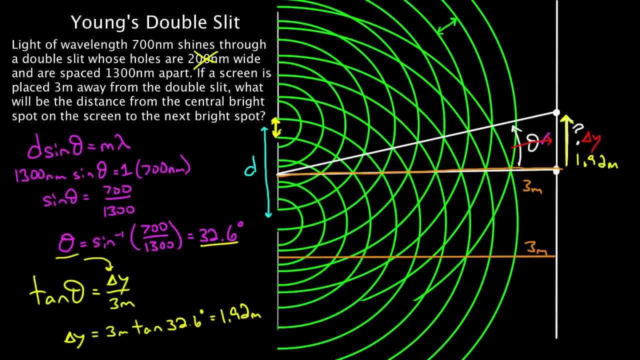 what would happen if we reduce the distance between between the slits? What would happen if we take this distance between slits and we make it smaller, We scrunch these together? Would this angle get bigger or smaller? Well, mathematically, let's just look at it. 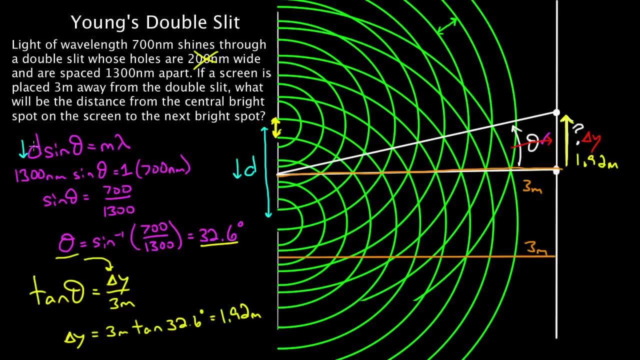 If the distance over here goes down in our formula, if D goes down, notice I'm not changing the wavelength. That's determined by the laser I fire in here, and this wavelength's staying the same. So this whole side's gotta stay the same. 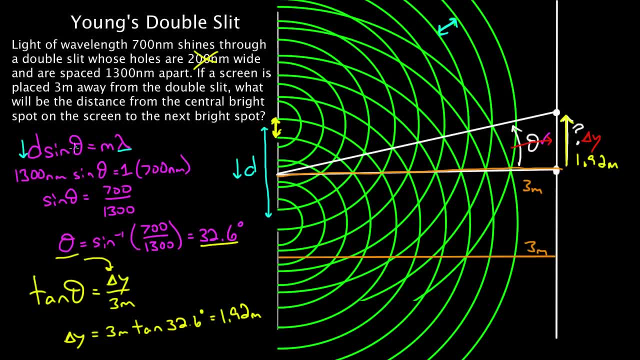 because M is still one at this point. So what's gotta happen to theta If the D goes down and the whole thing has to remain the same? the angle's gotta go up, because sine of a bigger angle will give me a bigger number. 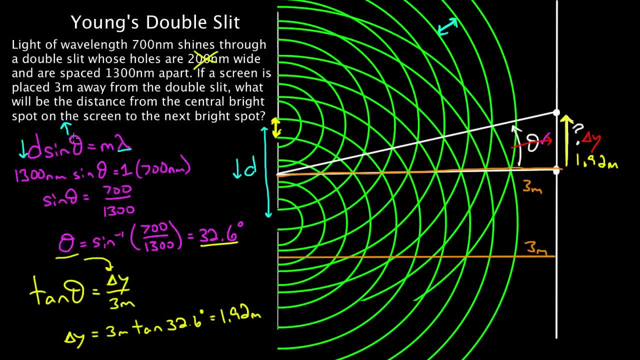 Sine of zero, zero, Sine of something bigger than zero gives me something bigger than zero. and the bigger the theta, the bigger sine theta. So as D decreases, sine theta's gotta go up. That's mathematically why. but I can show you in here: 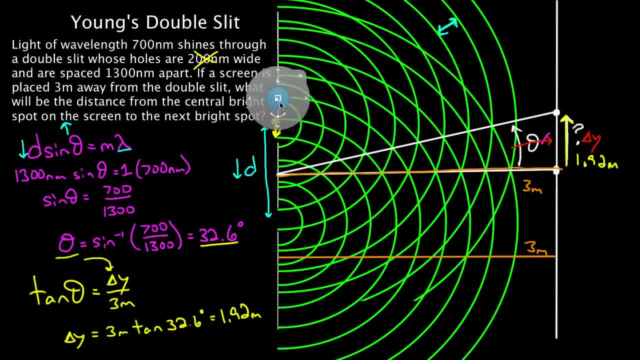 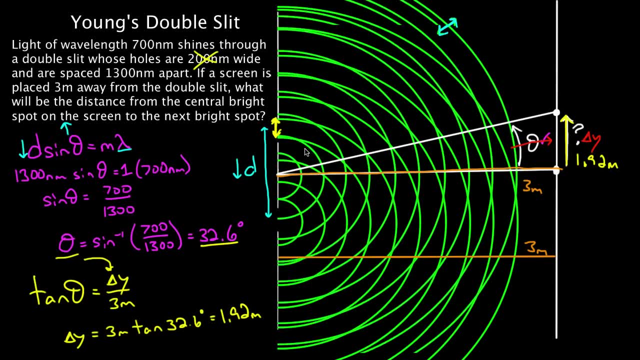 Check this out. Let's just take this. Let's take this here and I'm gonna move this whole thing down and watch what happens. Can you see the shadowy lines spread out? See how they're spreading out? And then we come back together.